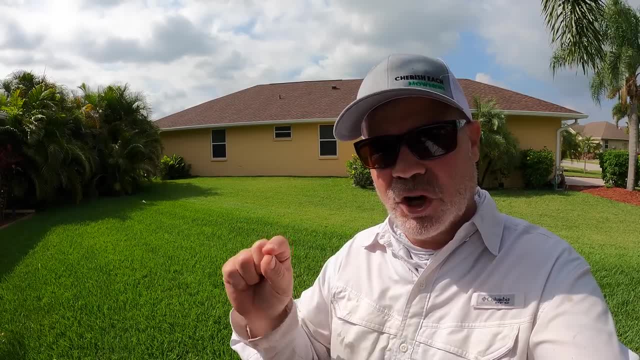 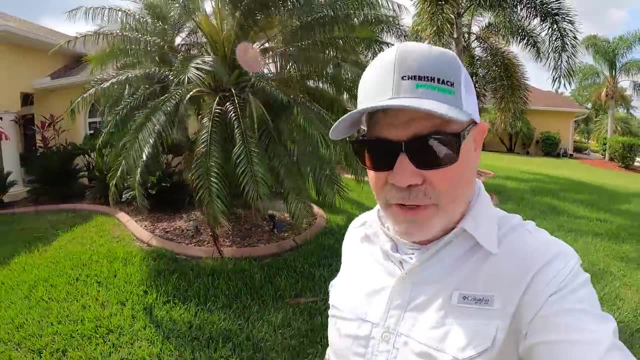 summer, but right now is peak, beautiful, dark, blue-green time for you. cool season grass pretty much anywhere in the country and, interestingly enough, when you get down, say, into Georgia, where folks are growing Bermuda grass, Bermuda's actually a lot slower to wake up than what you. 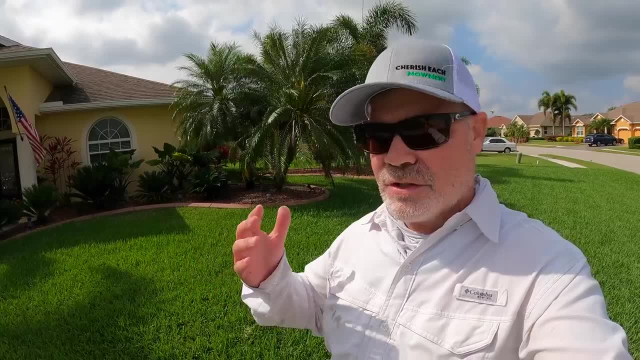 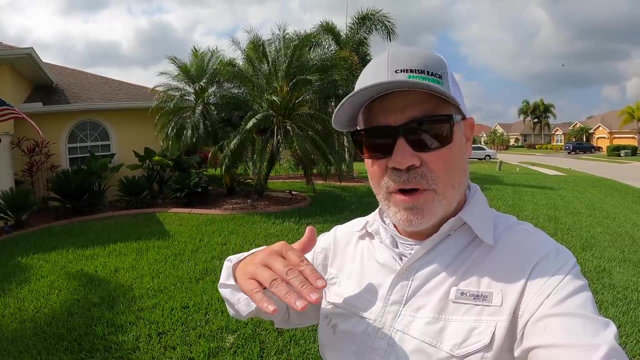 guys think I've talked about this before. With Bermuda grass, it isn't necessarily the heat that is needed, because there's plenty of heat With Bermuda grass. what it needs is longer days, and we are now at that point where the days are long enough. I don't. 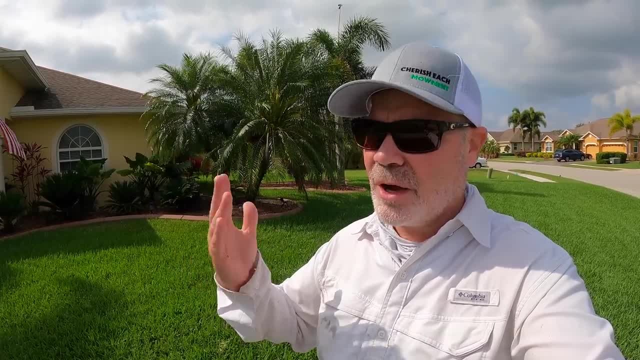 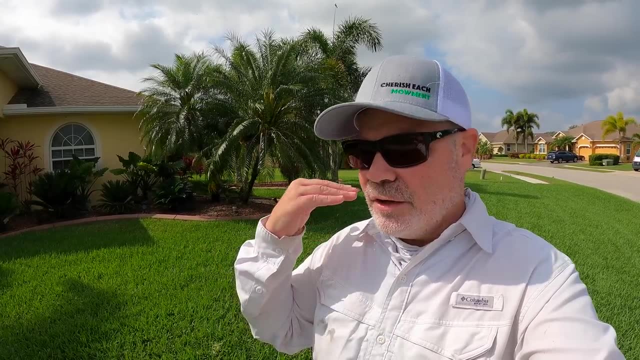 know about where you live, but here the sun is setting well after 8 pm now. Well, not well after a couple minutes after, but a couple minutes after 8 pm now, which means the days are much longer, and even the Bermuda grass, which is the most alpha of all but is also the slowest. 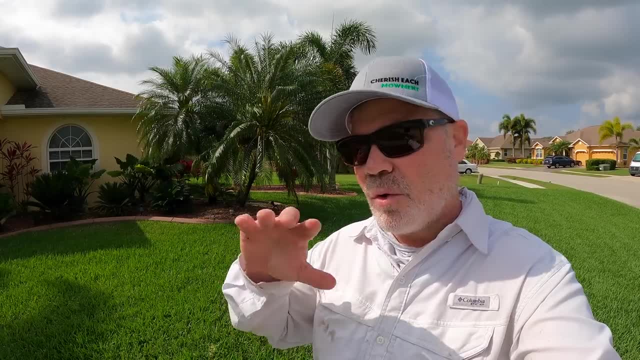 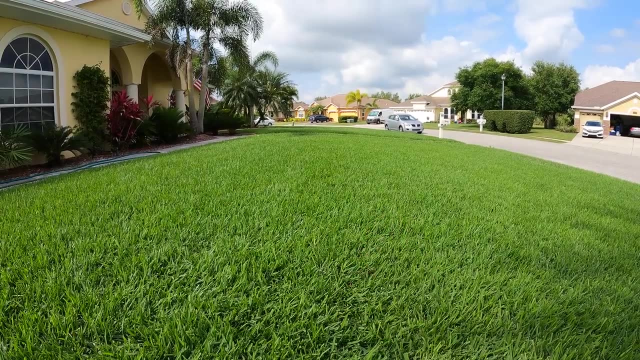 to wake up. even the Bermuda grass is raging in Georgia right now, or I should say it's about to peak. You get what I'm saying right. This is a time of unity For all of us. Of course, down here in Florida, my St Aug has been looking beautiful for several. 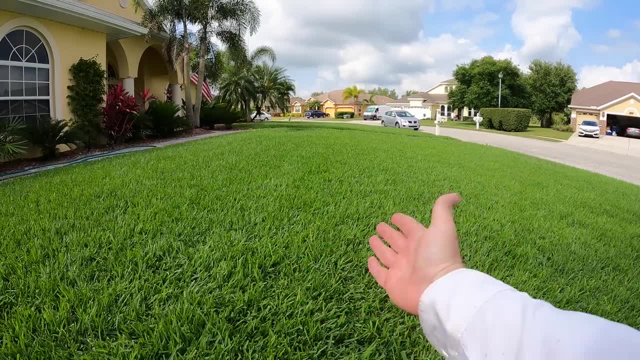 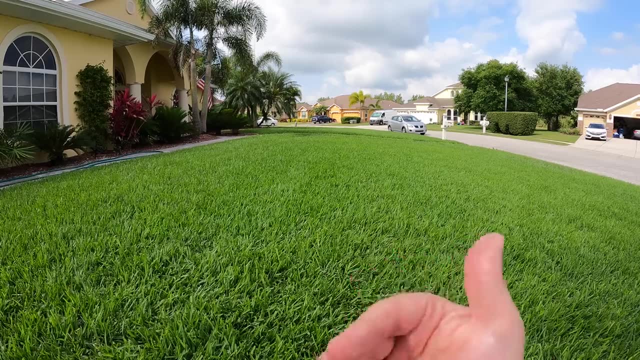 weeks, several months, Well, year-round pretty much. but you can see- and I don't know if you noticed, but in last week's video it was looking a little needy. and that's just me understanding my lawn. You know, after you do this for a while you kind of learn when your lawn needs something. 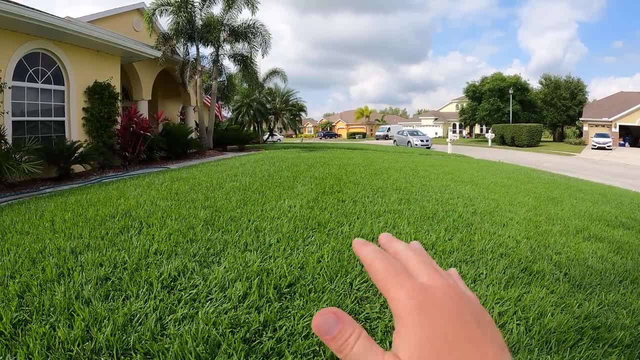 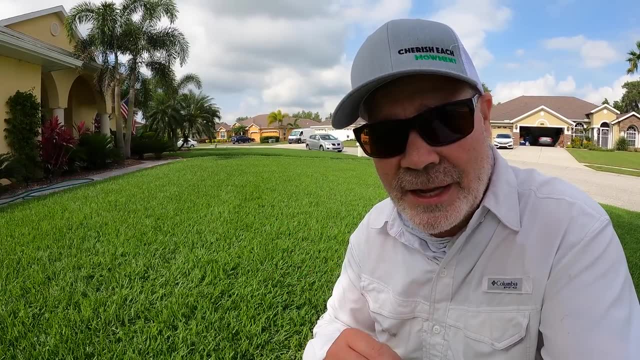 when it doesn't, You can just sense it. It's like any relationship: You just know when it needs something and you give it what it needs to keep the relationship in line. Do you mean to tell me your lawn reacts very much like your wife and other relationships in your world, son? 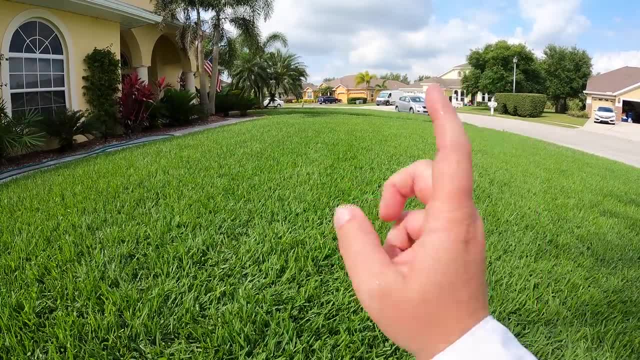 That was supposed to be Dr Phil, but it may have come out as Hank Hill, and I'm going to show you exactly how I did this, or really how you can do it at your house, And when I say that I'm going. 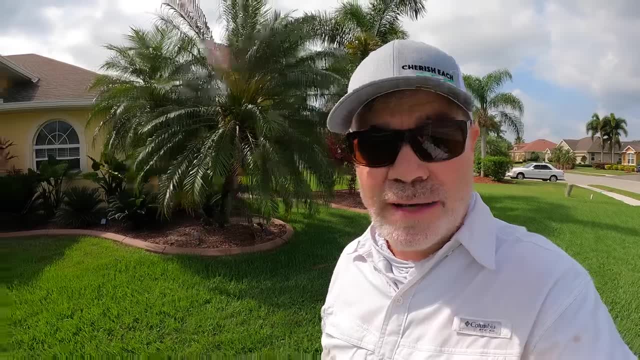 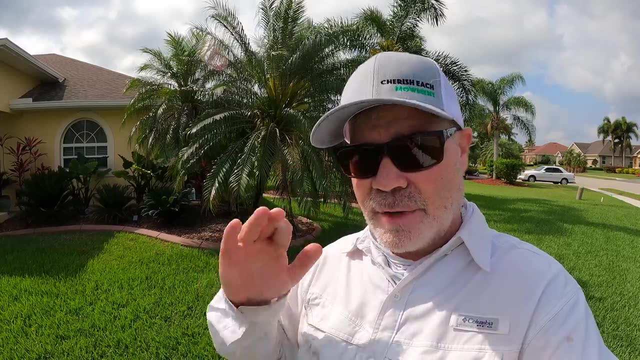 to teach you the three primary elements that you need to look for in any fertilizer, not just the ones I sell, Of course. I'll link those below, because that's what I do, but you can take the information that I'm going to teach you in this video. go to any store and find the three elements. 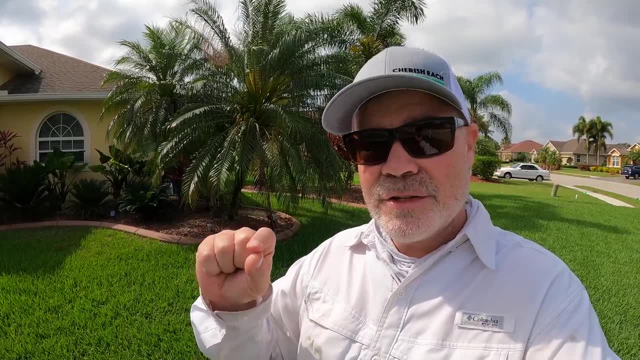 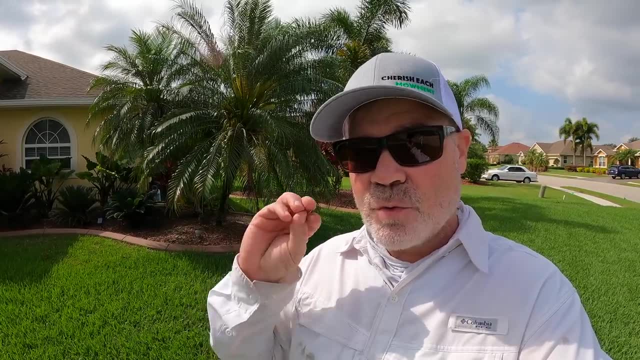 that I'm going to talk to you about today, that turn the lawn green, And the idea here is that, just because this is May 1st, we also have another very important day coming up at the very end of this month, and that is Memorial Day. Memorial Day is one of those days when you really want to have 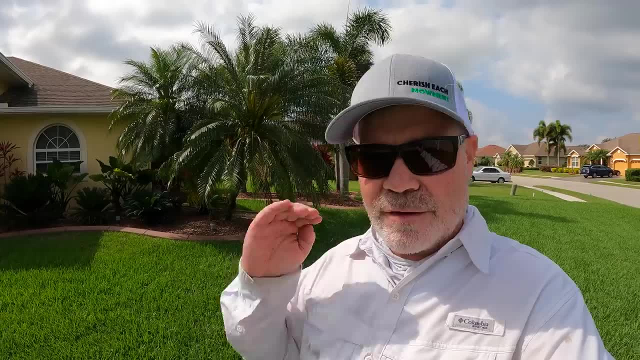 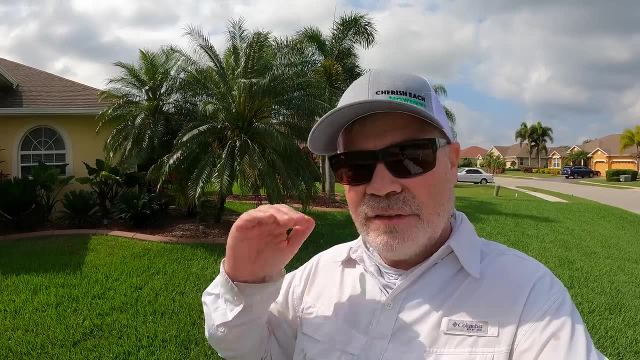 your lawn shining. If May 1st Derby Day, is an awesome day- one of my favorite days, Memorial Day is one of my other favorite days, second favorite days. Think of it like the one-two punch of May. I'm going to teach you how to do the one-two punch in May to get your lawn as green as possible. 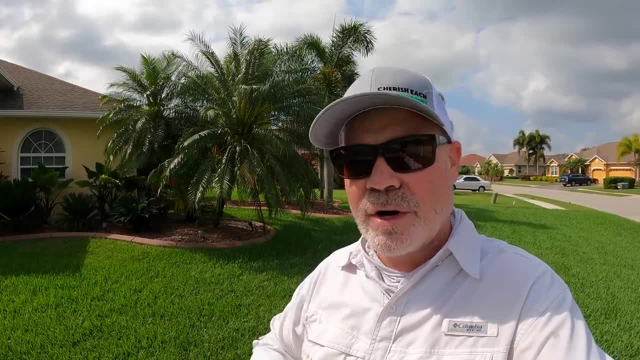 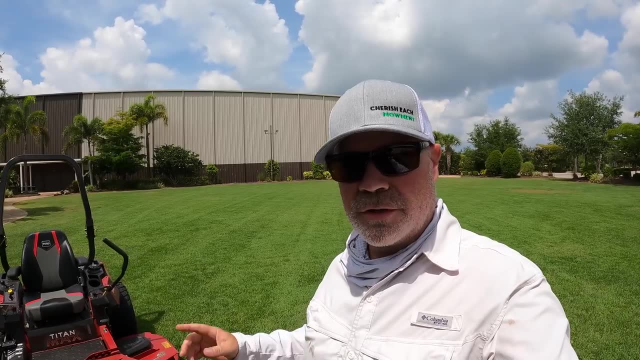 and now is the time to maximize it, no matter what your grass type, No matter where you live. Rattled that one off Too many cigars lately, All right, so I wanted to stop over here for a second. This is my project: lawn Zoysia. 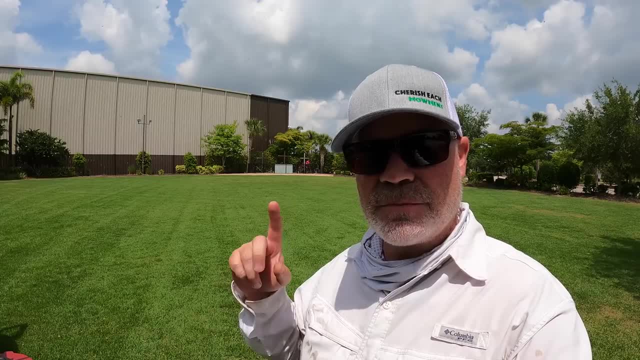 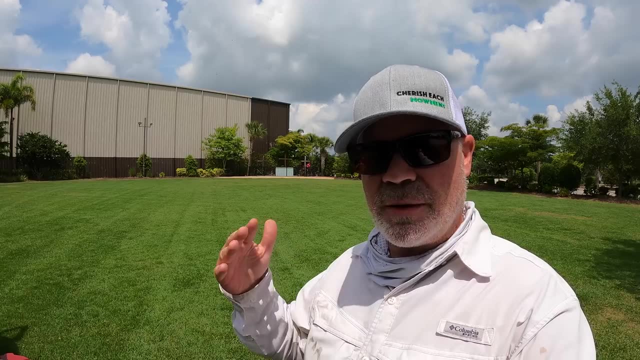 and you can see how green this is, and I'm going to tell you exactly how this got so green, and that is mostly because of nitrogen, and that's what this particular lawn needed. for sure, Zoysia, just like Bermuda, is a little bit slower to get going, even though down here in Florida. 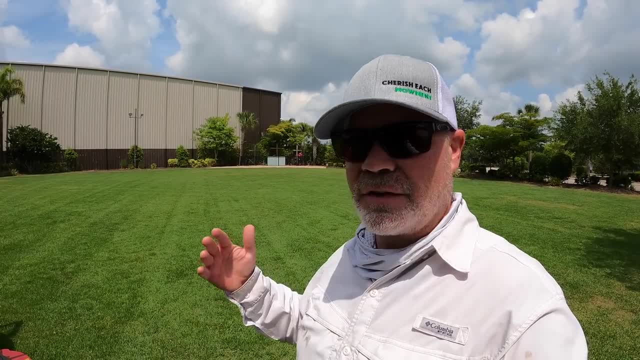 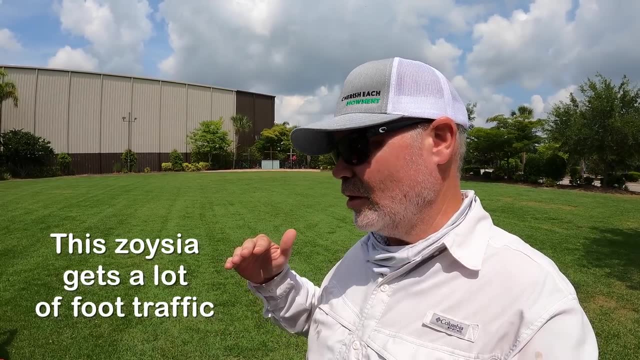 things are still plenty warm and we have long days and all that kind of stuff. But at least this Zoysia here I have noticed it just needs a little bit harder kick in the pants and I started it slow. I like to do that. I started with higher potassium, which we'll talk about in a minute. 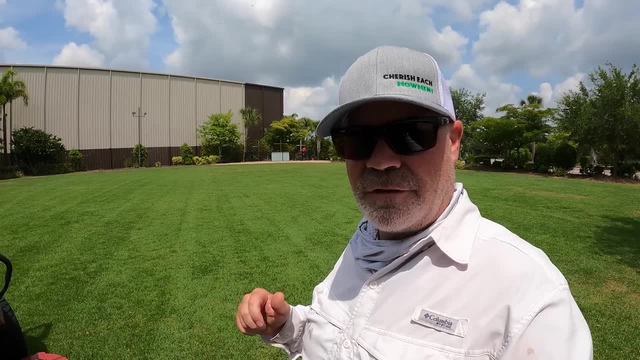 but I decided, now that the days are longer, it's time to start kicking it in the face with some nitrogen, and that's what I did. Now I'll tell you the lawn isn't perfect. This didn't make it perfect. 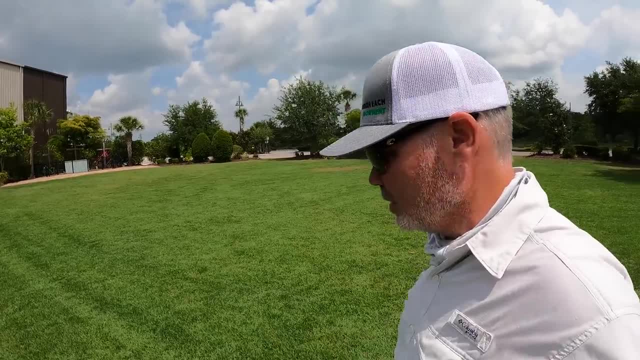 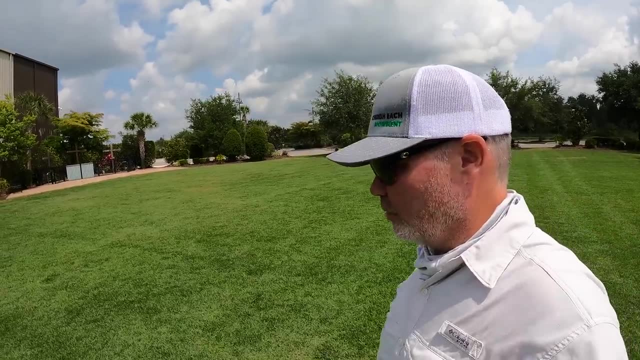 It had some disease challenges, which it still does. I've stopped the disease, and that's another thing. just a quick myth: People think that nitrogen causes disease. I'll link up there in the i to a video where I talk about it. 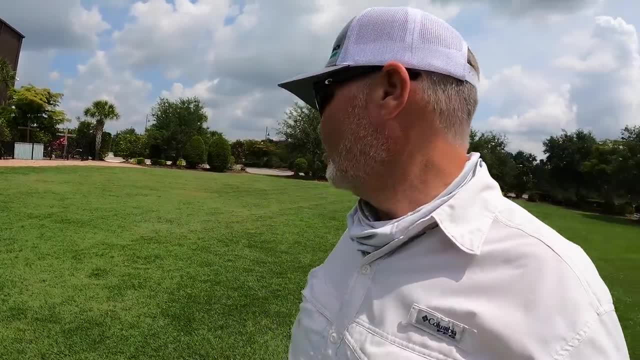 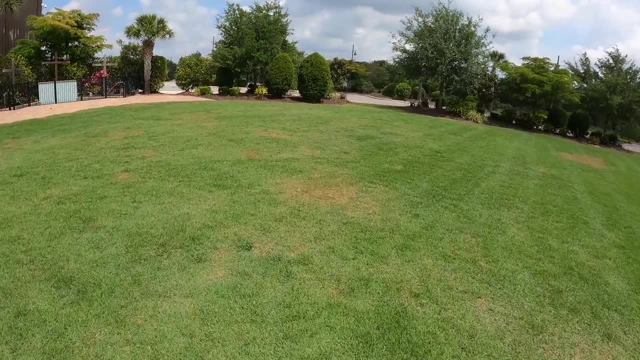 because that's somebody reading university websites incorrectly. but you know you can see the place where the disease scars were. They're not cured. I mean, that's the whole thing. Nothing cures areas that have died back from either disease or insect or whatever. 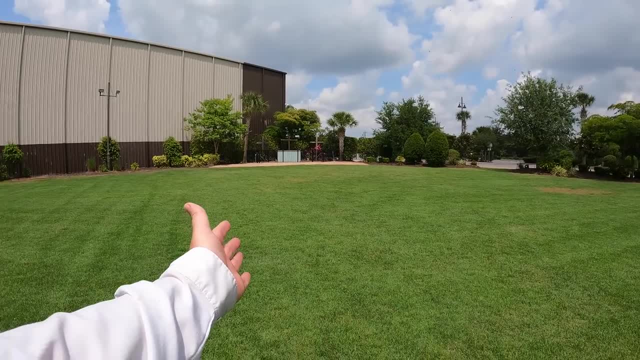 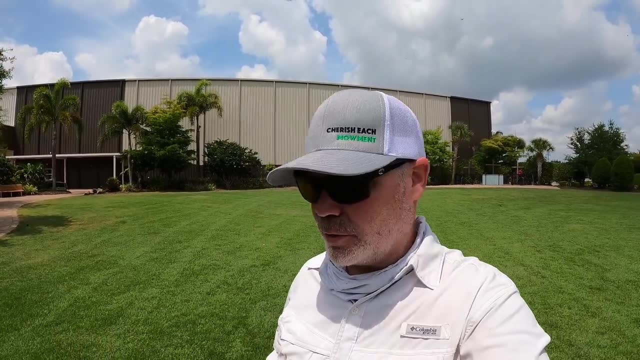 Those are going to take a little bit longer to come back, but what you can see is that, overall, the lawn is looking better, and that is because I put down nitrogen. So nitrogen is the first number on the bag of fertilizer. so whether you go to the store or whether you get what I link in the description below, 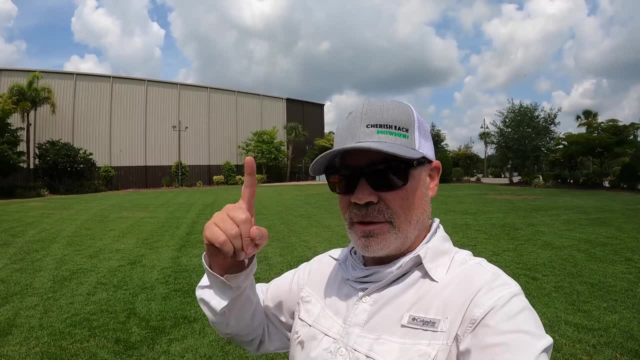 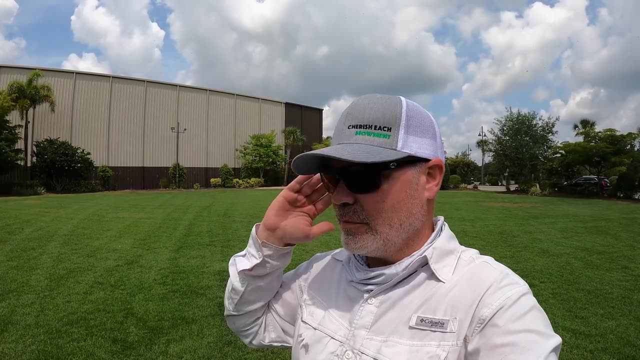 the first number. when you see three numbers on the bag of fertilizer, the first number represents nitrogen and this time of year, right now, May, when we're all running fast, you want that to be higher. You definitely want that to be up somewhere north of 20.. 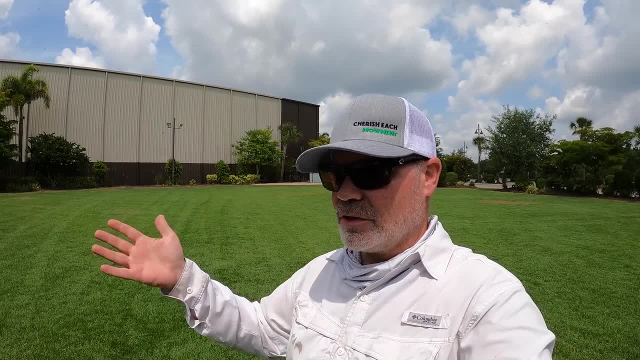 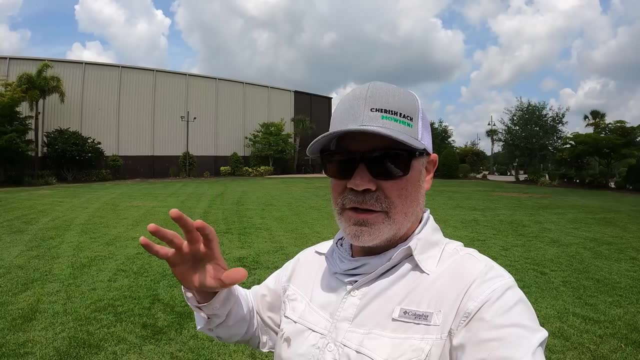 Now there's some different ways that the nitrogen can be delivered. Some of it can be slow release, Some of it can be immediate release, and even those terms are a little bit suspect but they don't necessarily describe what it is. but the long and the short of it is: if you make sure you get a product and again, if you want to go to the store and get it, please do. 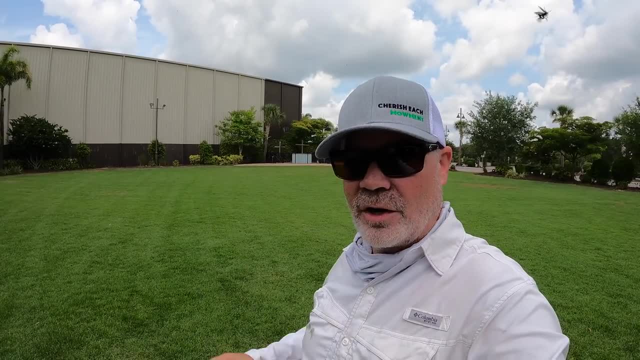 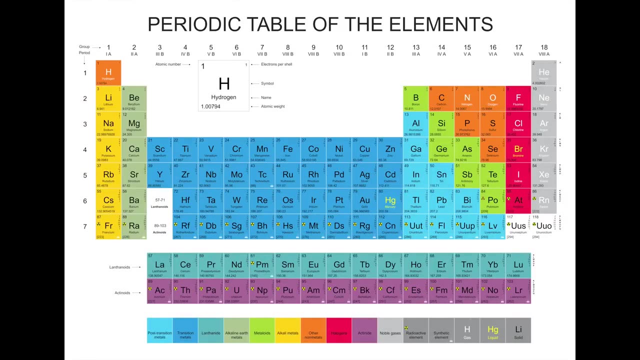 something that is higher in nitrogen, you're going to see better results quicker this time of year. Out of all the elements that we find in fertilizers, nitrogen is the most important. As I have often said, nitrogen drives the bus. All of the other elements ride along on the bus, but nitrogen is what drives them. 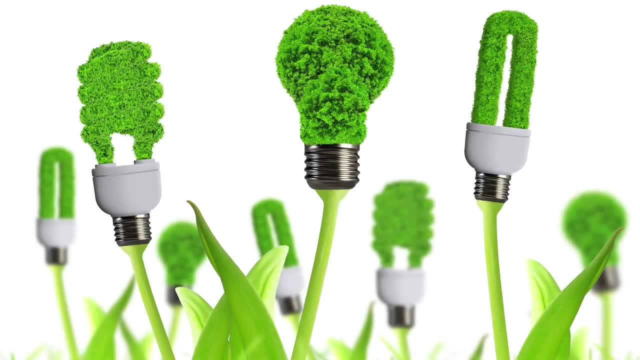 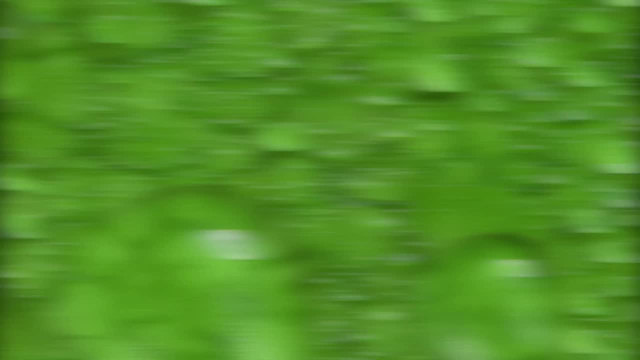 When it comes to the overall look of the lawn. it's nitrogen that gives grass its basic green color, and that's because nitrogen makes up a large part of chlorophyll. Chlorophyll is the green part of the leaves and the stems that you see. 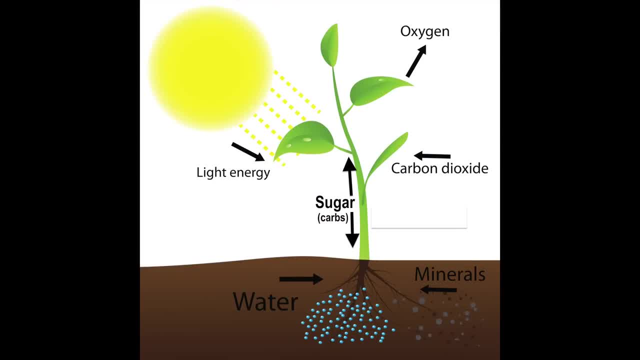 Light energy is taken in by chlorophyll. Chlorophyll is used to make sugars for the plant. We call this photosynthesis. Nitrogen is also very important when it comes to regulating plant growth. The more leaf surface the plant has, the more sun it can absorb, and of course that makes sense because that makes the grass thicker. 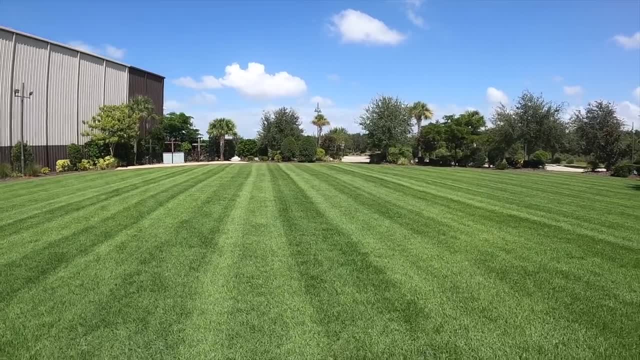 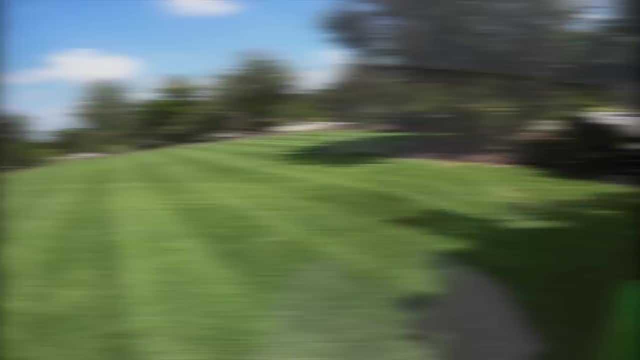 Never forget: nitrogen drives the bus. If you want a green lawn, you'll have nitrogen in every single application you make all year long. So nitrogen is the first number on the bag of fertilizer. So whether you go to the store or whether you get what I link in the description below, 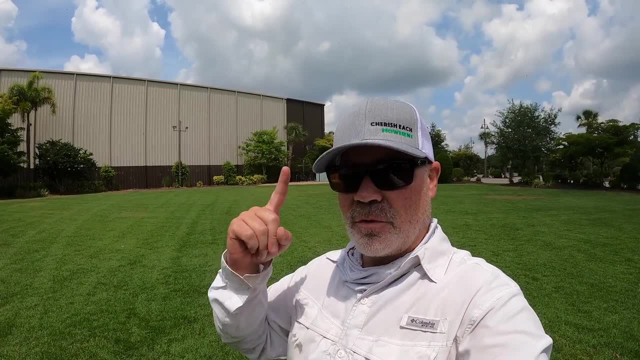 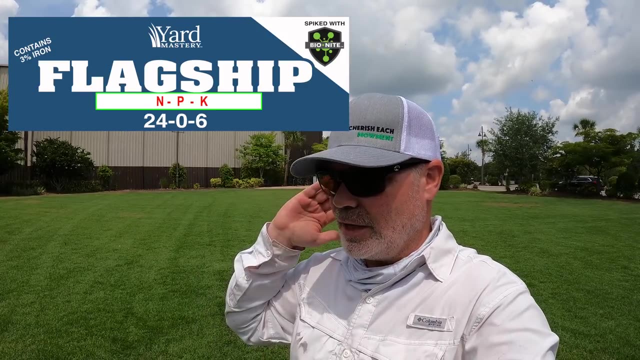 the first number. when you see three numbers on the bag of fertilizer, the first number represents nitrogen And this time of year, right now, May, when we're all running fast, you want that to be higher. You definitely want that to be up somewhere north of 20.. 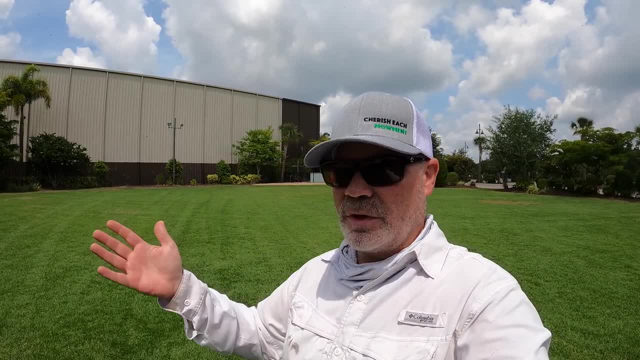 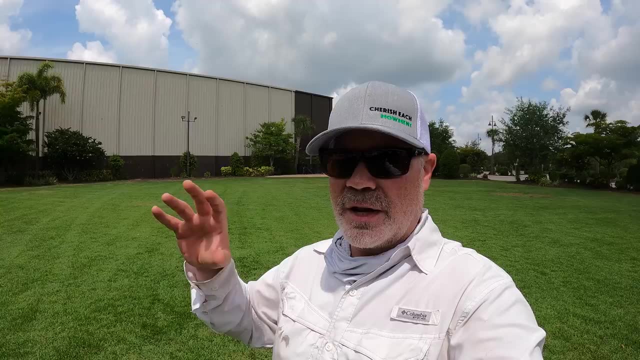 Now there's some different ways that the nitrogen can be delivered. Some of it can be slow release, Some of it can be immediate release, And even those terms are a little bit suspect but they don't necessarily describe what it is. But the long and the short of it is: if you make sure you get a product- and again, 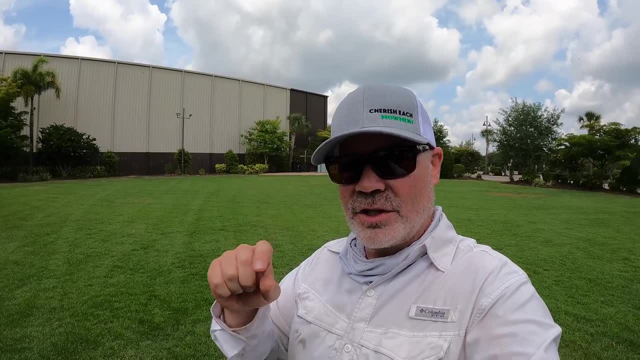 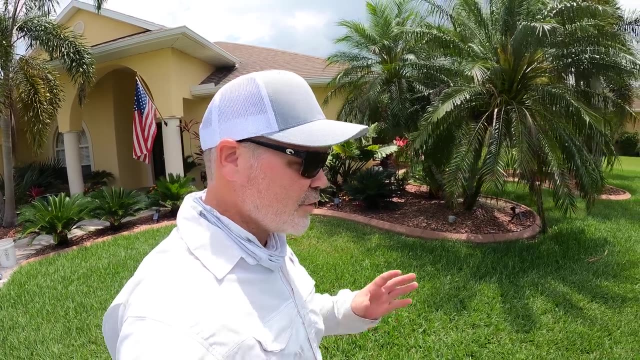 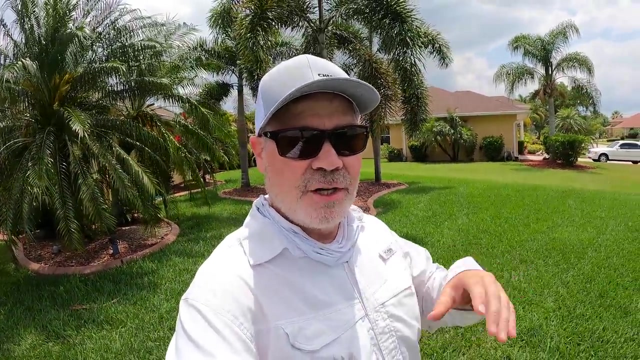 if you want to go to the store and get it, please do something that is higher in nitrogen. you're going to see better results quicker this time of year. Okay now, the second element in the fertilizer that you want to look for that's going to help you get the greenest grass possible is potassium or potash. 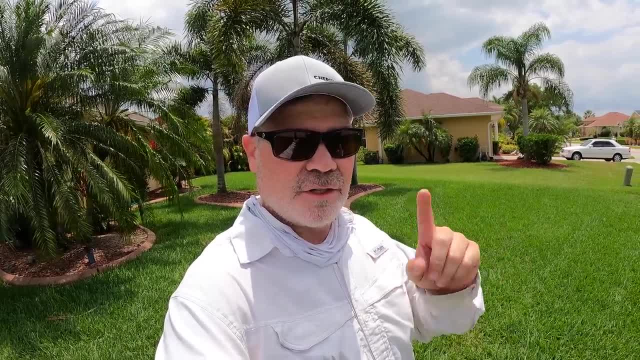 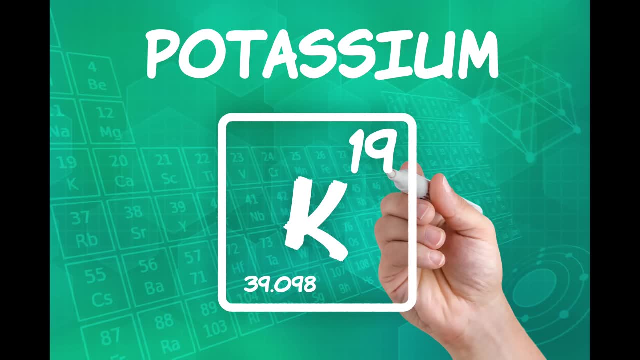 Potassium does a lot of things for plants, a lot of things for lawns. Let's go over those real quick. The next element that you're going to want to look for in any fertilizer you purchase is potassium, When you look at the three numbers on the bag of fertilizer. 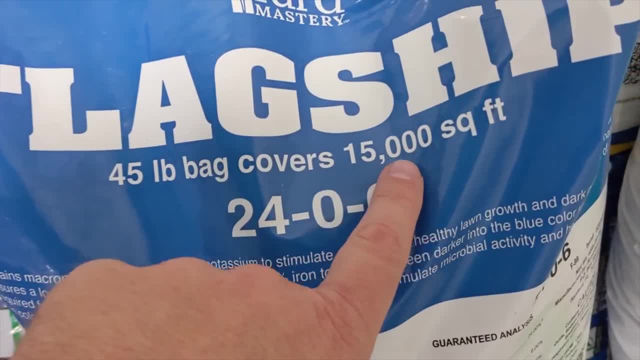 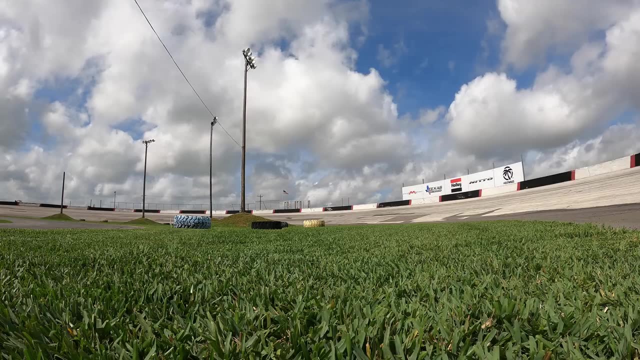 potassium is the third and you're going to want this to be well above three or even four, if you can find it. The long and the short of it is: potassium reduces stress and a stress-free plant can be greener and taller and healthier and look more vigorous. 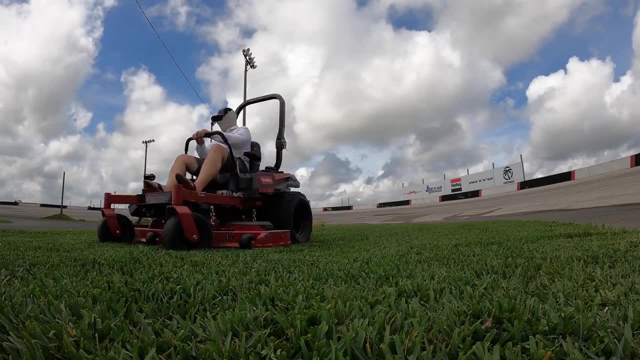 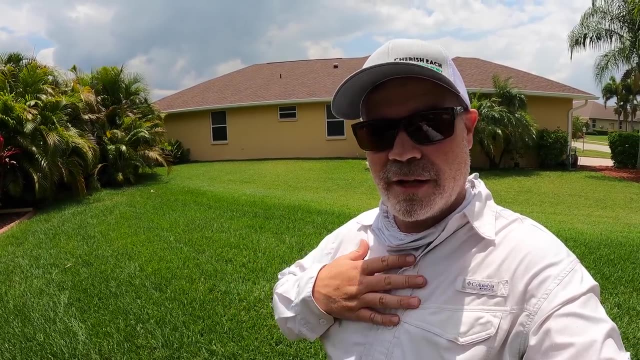 which means it will dominate the stressed out lawns of your neighbors. So you can see, potassium is extremely important, but one of the things that I like about it- again, we're DIYers, we have to have the visuals too, and that's part of what, all of that, I teach. 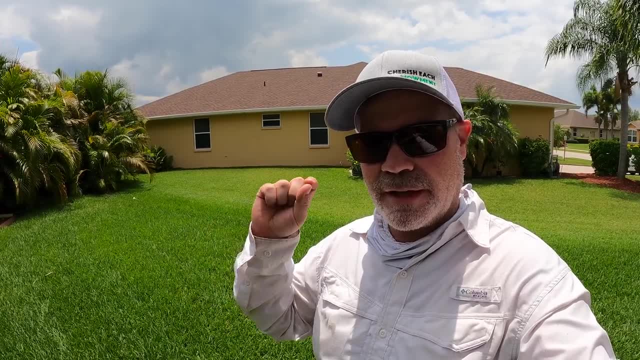 I want you to get a healthy lawn, I want you to get healthy soil, but if I can help you get visual results along the way, then you're going to go further, You're going to go deeper and you're going to want to explore more and learn more. 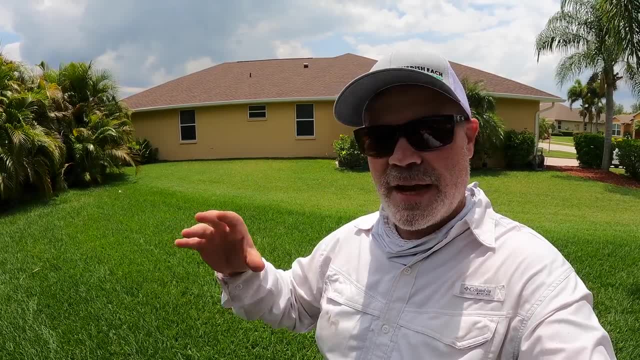 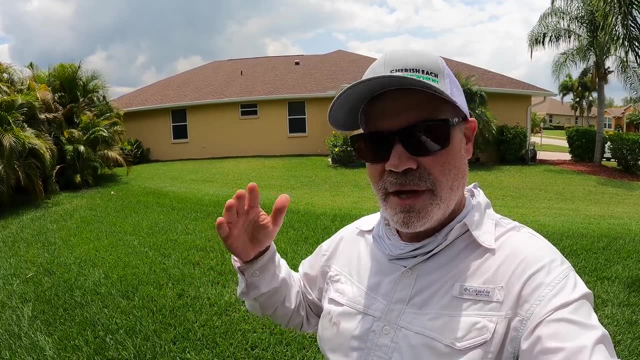 but I got to get you the visuals first. That's just how the world works, right? So potassium is another one of those. when it's higher in your fertilizer, it's going to give you a green color, And I've always said for many years that potash or potassium, gives your lawn a truer green color. 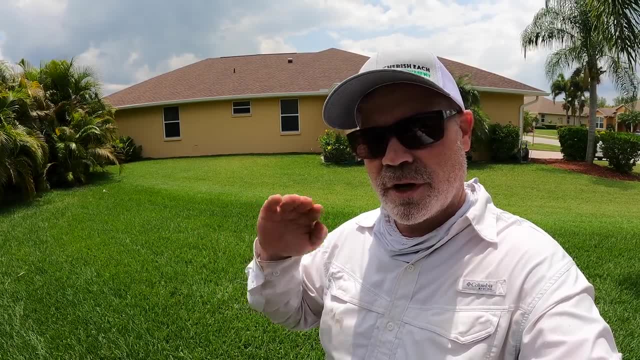 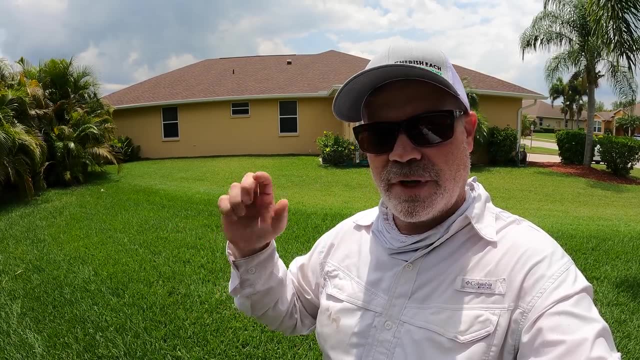 And that's really nice because it's that bottom end green, that nice truer, truest green, not hunter green, but just that truest green color, that base layer of beautiful green. That's what potash does when you put it down. 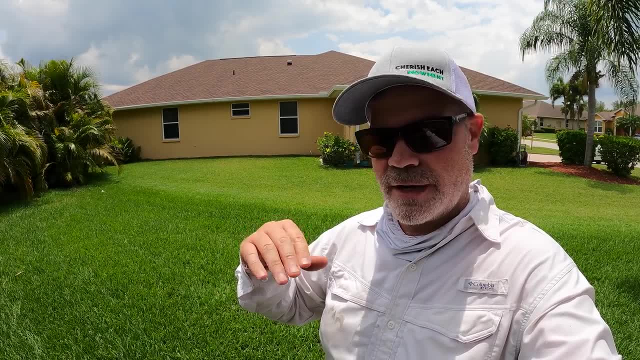 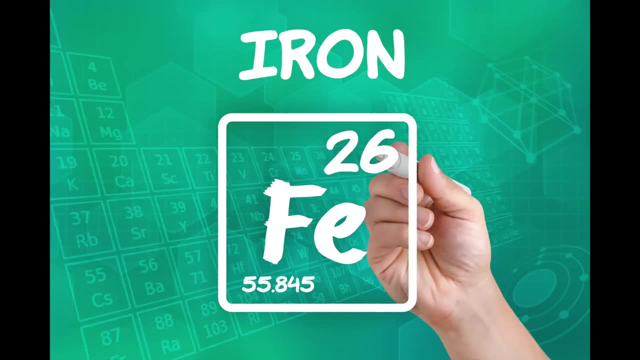 Now I actually have fertilizers that are higher in potassium and a little bit lower in nitrogen, and they get great results too, but only because they also include the third element in our list. Now, when it comes to iron, we're going to mention a familiar term we've mentioned before, and that is chlorophyll. 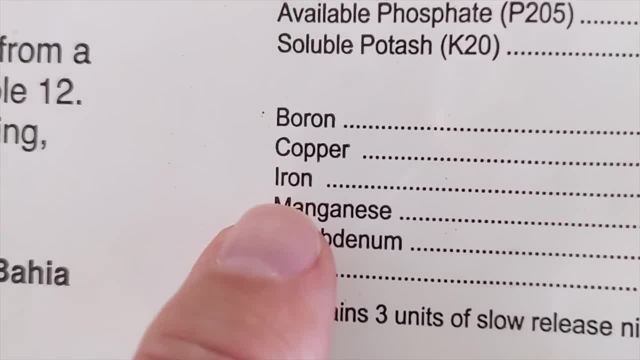 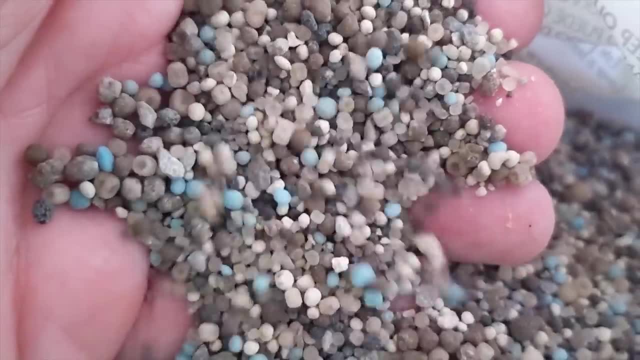 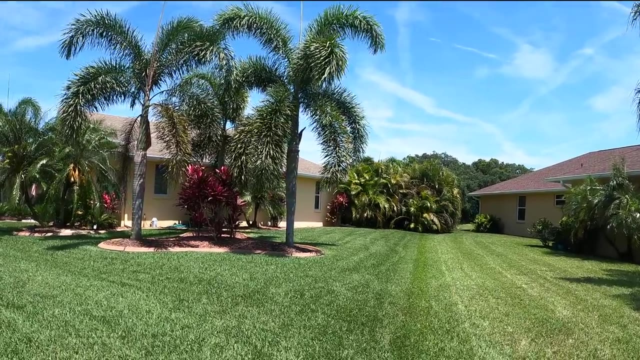 Iron is directly involved in the manufacturing process of chlorophyll and is required for many enzyme functions in the plant. The biggest reason we, as DIYers, prefer iron in our fertilizers is because it's what gives your lawn the deeper, darker blue-green color that truly dominates your neighbors. 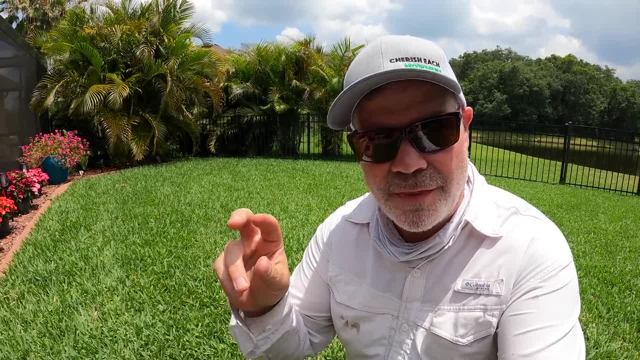 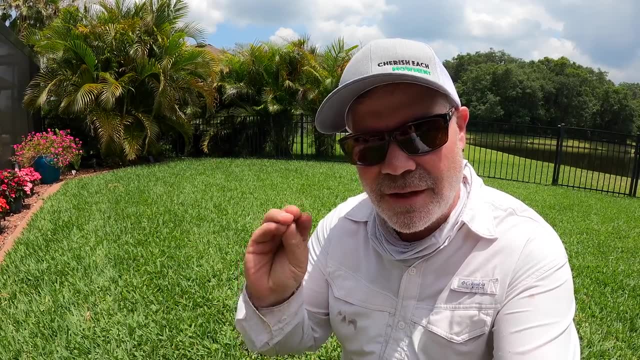 So iron is what gives lawns that blue-green color and that kind of balances out: the bottom end green that you get from the potassium, as well as the straight up green and sheen that you get from the nitrogen, When you find a fertilizer that has all three of those in it. 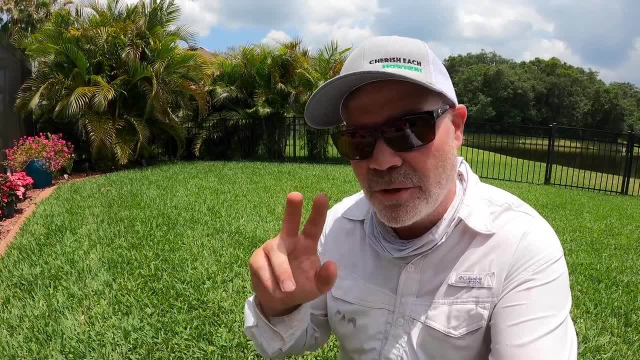 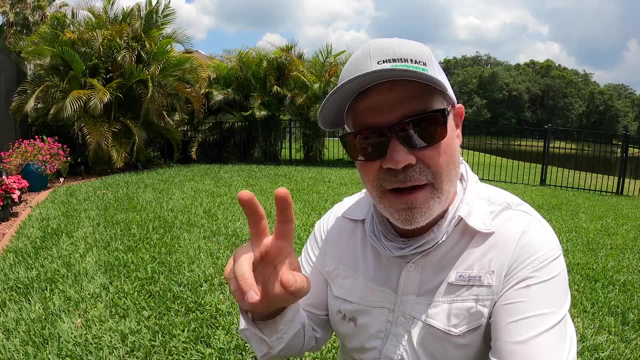 you are going to get results. You're going to have a greener lawn within a few days after the application. Now here's the thing: each time you see these elements and there's a number on the bag, that number stands for the percentage. 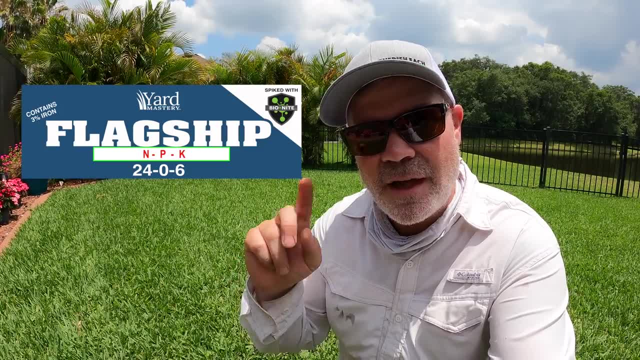 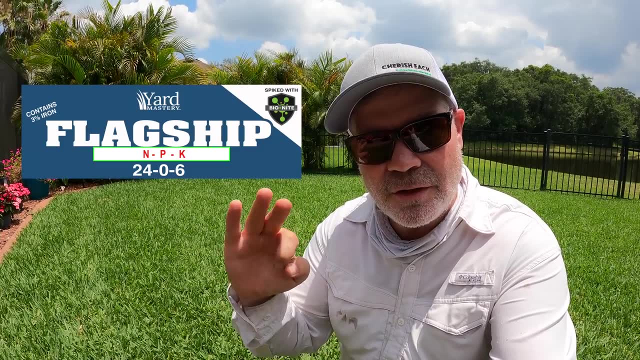 So, for example, in this fertilizer here at 2406, that means 24% of that bag, everything in that bag is nitrogen, 6% of everything in that bag is potassium or potash, and then you can see here on the corner, 3% of everything in that bag is iron. 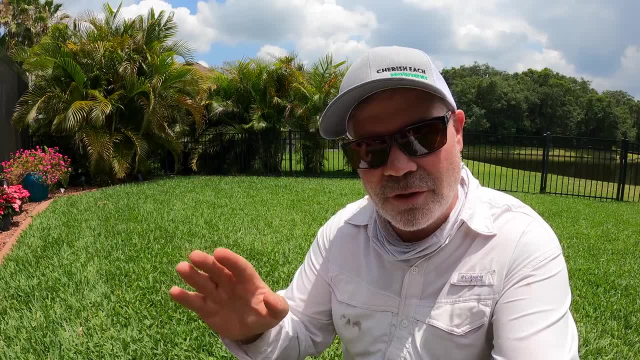 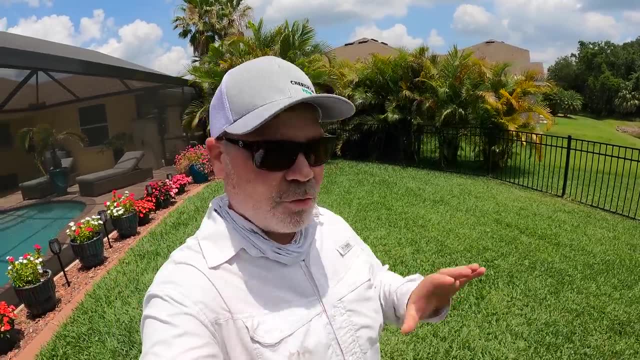 The higher those amounts, the greener. the greener your lawn should be. It's literally that logical and it is literally that simple to understand the results that you're going to get Now. I want you to keep in mind: We're talking about May applications right now. 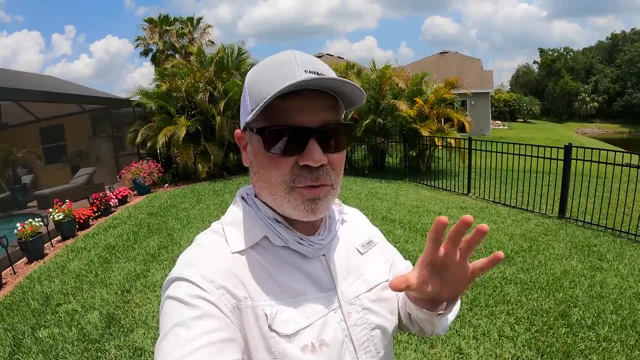 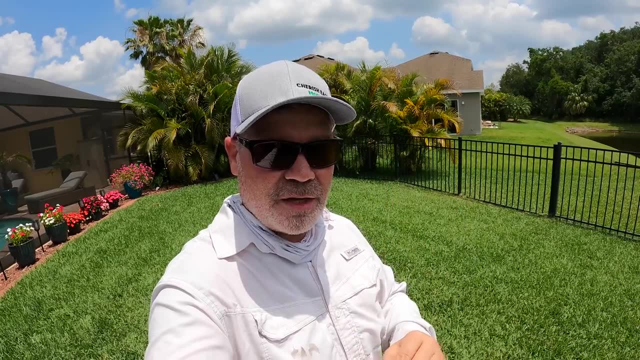 Every single one of you can use the same for right now, again, because of what I talked about in the beginning, We're all at Peak, or just entering Peak or what this back into the Peak, but we're all somewhere real close to the Peak. So higher nitrogen, some potassium and some iron is perfect for everyone right now. Now when you get to summer, things will change and if you subscribe to the channel here, I'll talk about that. It's an important free resource that you can get right now. 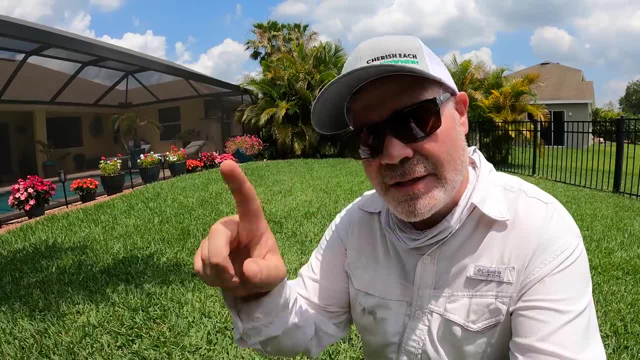 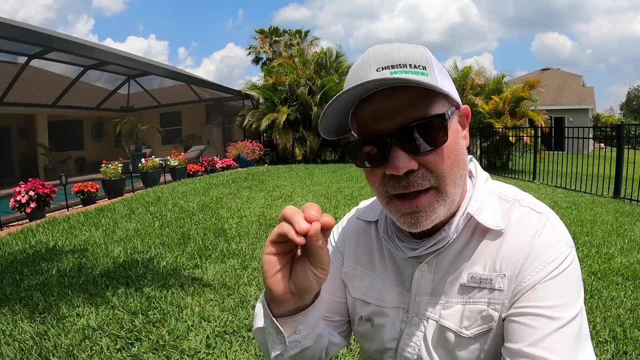 I'll link it below. I just wrote a guide on how to read a soil test, But as I go through that- how to read a soil test- I actually talk about the different elements that are inside of fertilizer and what they mean and how to understand that, how to interpret that fertilizer. 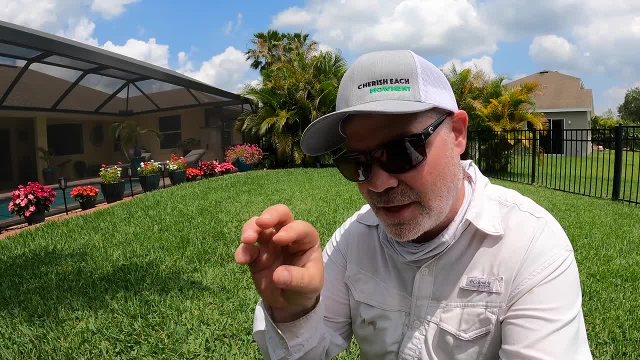 And even though, again, it talks about the fertilizers I sell, you can take that information that I teach you there and go to any store and apply it and get any fertilizer at the store that you want to, and I really encourage you to do that. 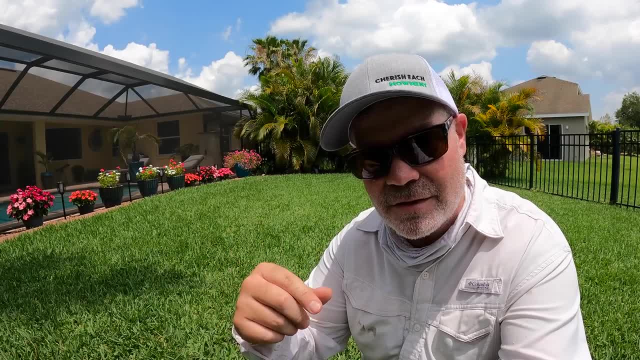 You don't have to give me any email address, nothing, It's just below. It's a PDF guide that's linked. You can just get it right now and download it, and I guarantee you'll come away learning something If you get that free guide on how to read. 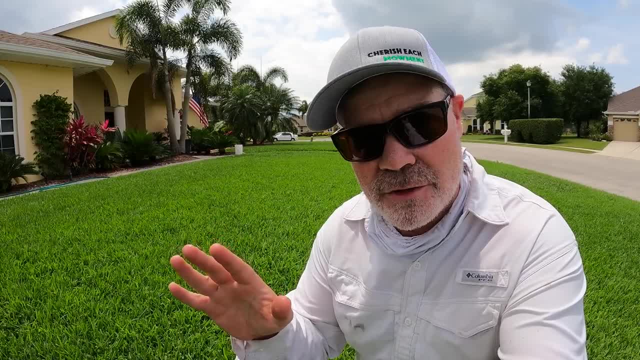 and interpret and set up a strategy based on a soil test. I'll tell you a little bit more about soil tests in one second and I'll be done with the video here. But a lot of you are going to ask: Okay, Alan, you showed us all this. the three elements. 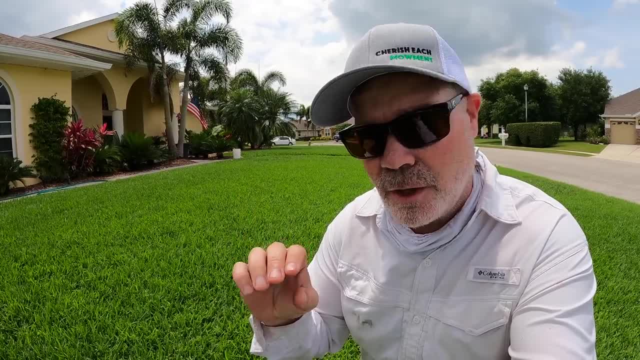 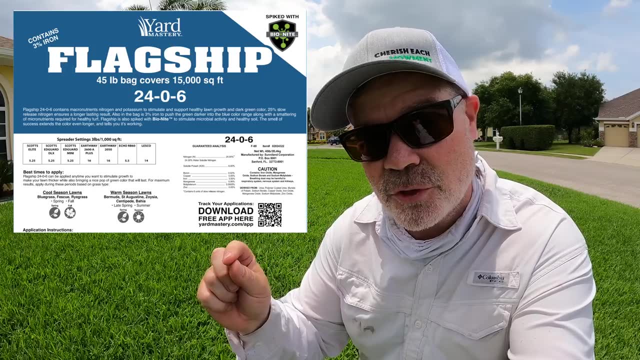 We need are nitrogen, potassium and iron. Where do I get that? Well, all of the lawns that you've seen here have been hit with my flagship blend, the 2406, within the last couple, two or three weeks. That is what has produced this color.